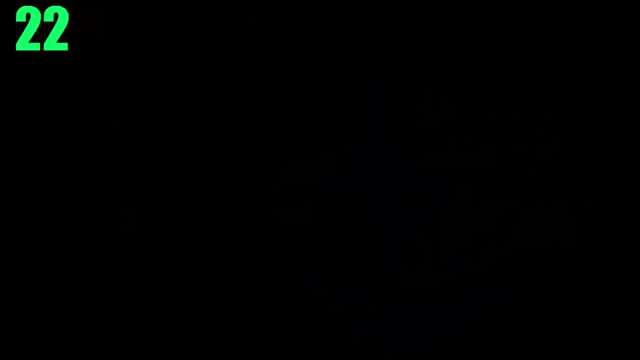 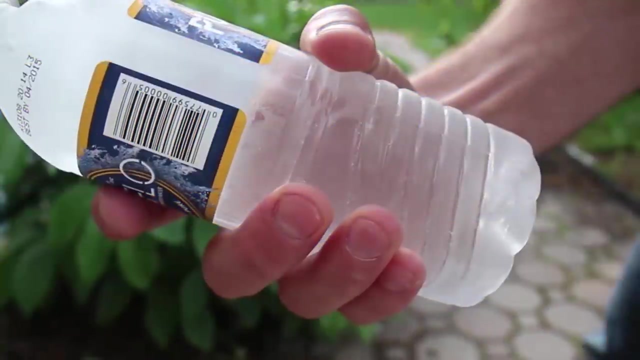 Number 22,: instant ice. Here's a simple way to get a nice cool water on a hot day. Take a water bottle and put it in your freezer for about two hours and 45 minutes, just before it would freeze into ice. Times can vary, though, for different freezers. At this point the water is well below. 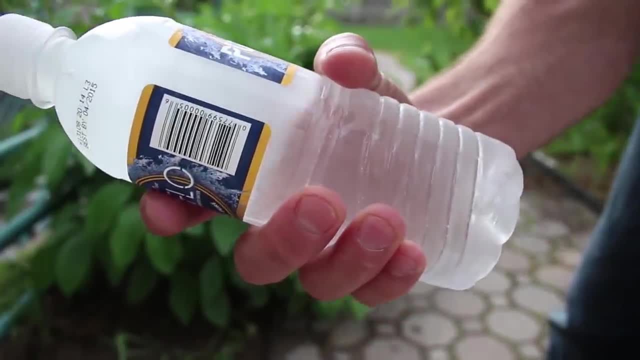 freezing and just needs some little bit of help. So with a nice tap, and there you have it. You can also gently pour it into a glass and dry it out. Number 26,: instant ice. Here's a simple way to get a nice, cool water on a hot day. Take a water bottle and drop a piece of ice into it with the 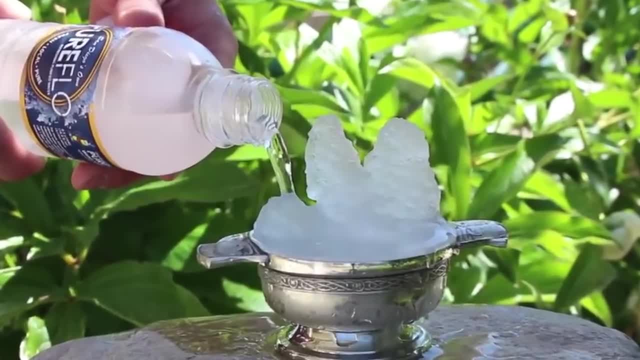 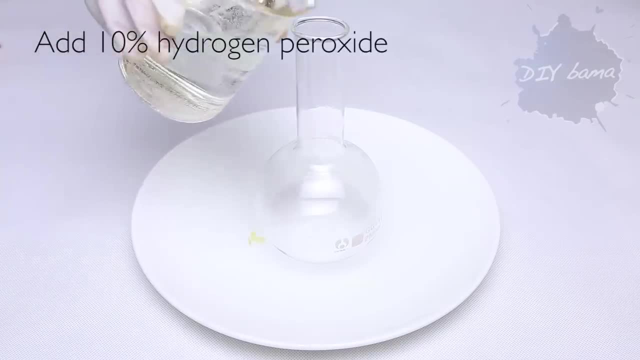 same results. You can also do this same trick with soda for a delicious, awesome result. Number 21, elephant toothpaste- Not literally. What you'll need to do for this experiment is pour 10% hydrogen peroxide- because this is a safe version- into a flask with a little bit of. 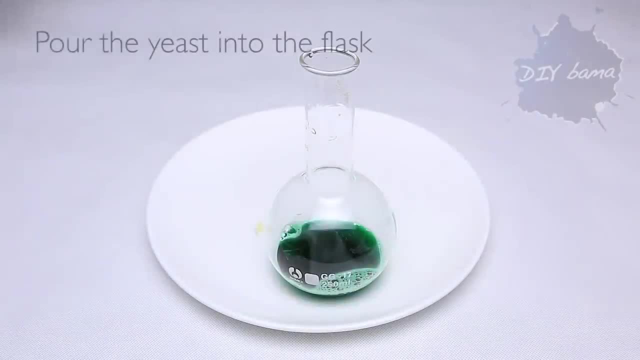 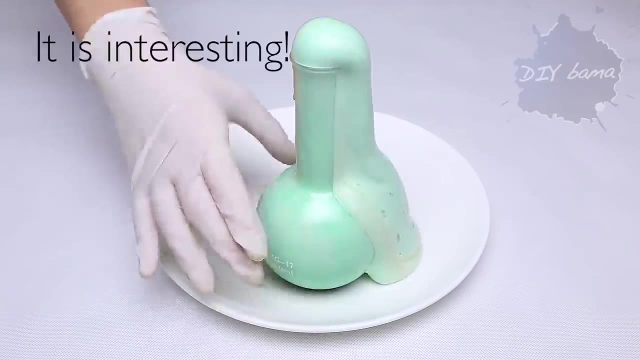 dish, soap and coloring of your choice. Then, in a separate container, mix yeast with warm water, Pour it into the flask and you've got yourself toothpaste for a lifetime. Number 20,: firebending Finally my dreams of joining the fire. 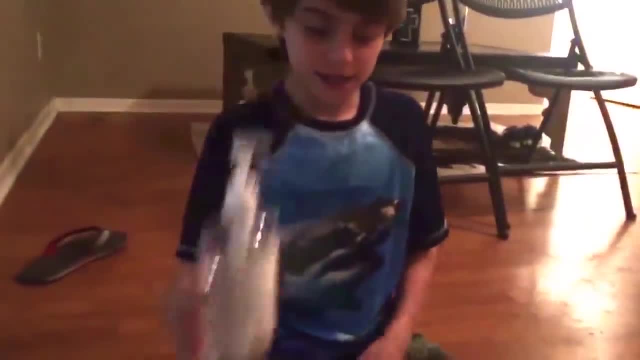 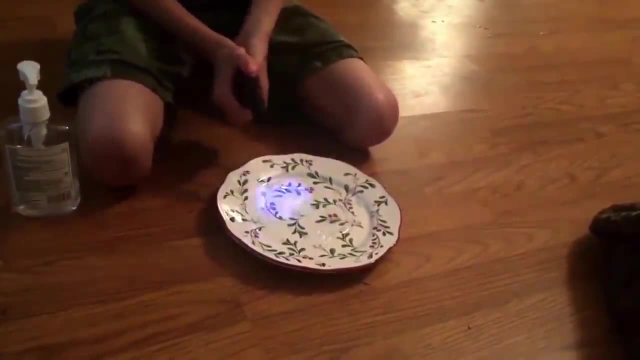 nation have finally come true. But on a real note, this one is extremely simple. For those of you who don't know, hand sanitizer is pretty flammable and just by lighting it again, be safe. don't actually try this. it will cause fire. But it's actually reasonably safe to grab and hold. 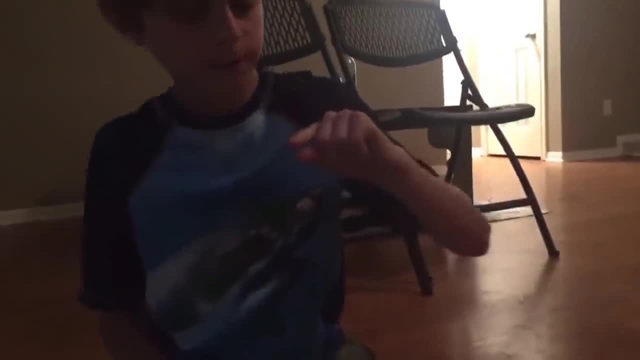 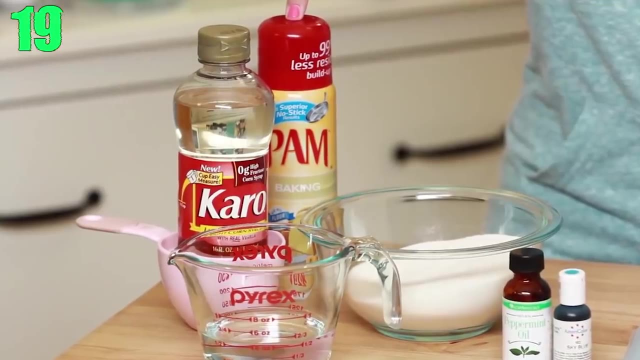 just not for too long, of course, and keep your hands in motion in to help. And also, again as a side note, please, if you do try this, make sure you have parental guidance and you're safe about it. Number 19, glass candy. Here's how to make a delicious peppermint candy. What you'll 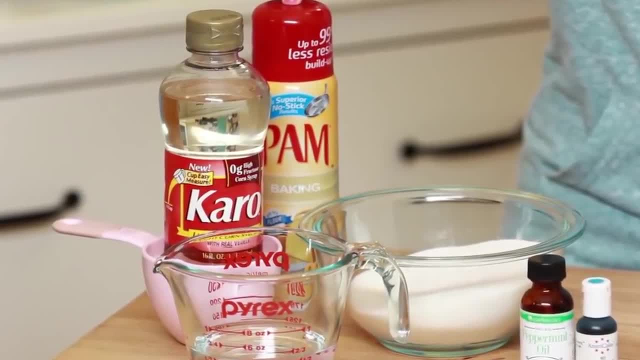 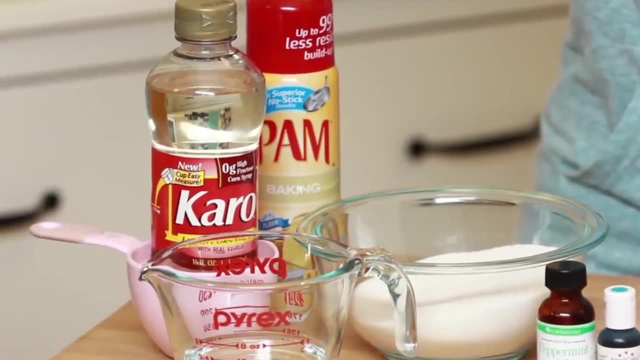 need is baking spray: two cups sugar, three-fourths cup of corn syrup, half cup of water and two tablespoons of peppermint extract. but really you can use any clear extract you like, But blue food coloring is pretty awesome. I would suggest blue. it's my favorite color. But anyways, cover up a. 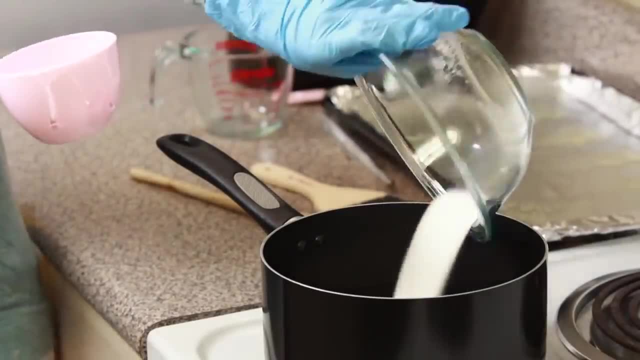 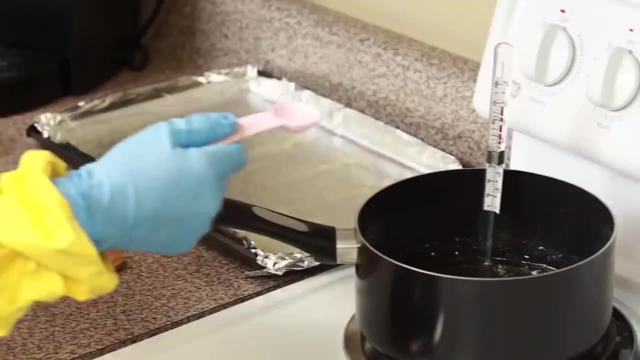 tray in aluminum foil. Next, fill a heated pot with your sugar, corn syrup and water until it's all liquefied at around 285 degrees. Also, make sure no sugar is on the side of the pot for the best results. Once boiled, add your peppermint extract and drop of food coloring and stir until 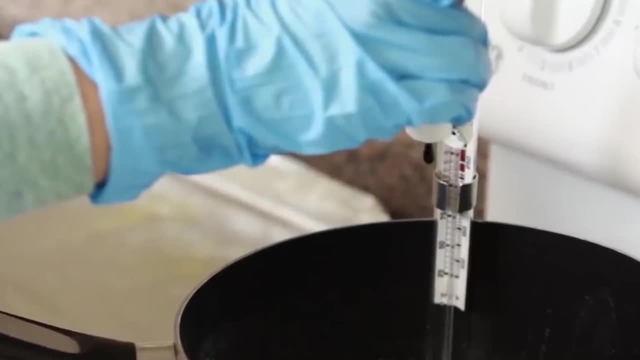 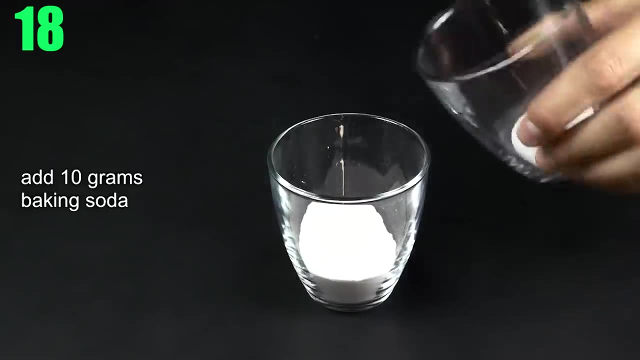 you get a nice color. Finally, add the baking spray to your aluminum sheet and pour it into your concoction in and then let it sit for about 30 minutes to harden. Break it however you wish. Number 18, fire snake. First, mix 10 grams baking soda to 40 grams sugar In a bowl. fill it with. 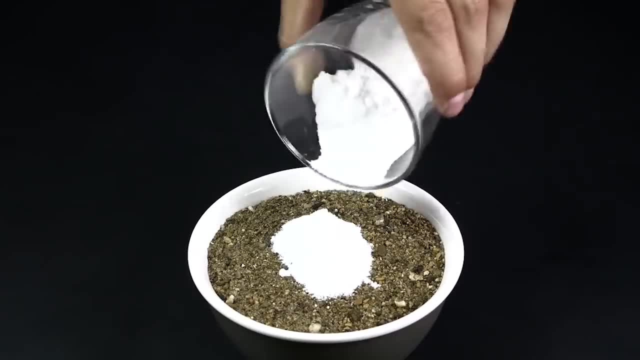 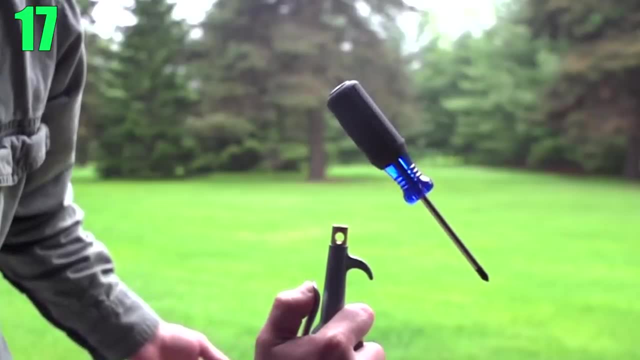 sand and pour lighter fluid into it, Pour the baking soda and sugar mix over it and light it up however you can. Honestly, it's wild and it just keeps growing. Number 17, levitation. What is this sorcery? Oh, just science and a little bit of luck. Okay, so if you have access to an 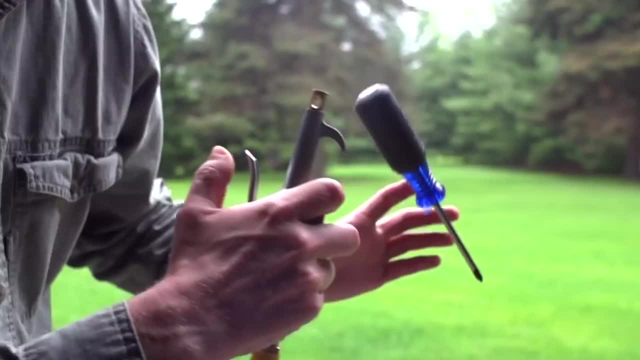 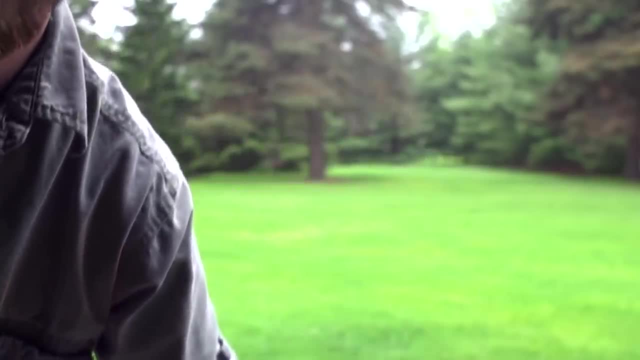 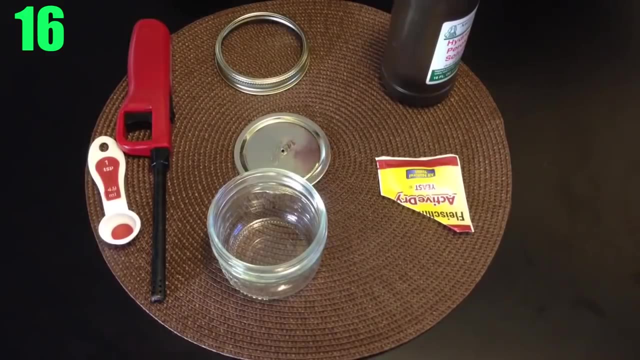 And just try to find the right angle where it'll float. It's simple, but it's also difficult, So on that note, good luck. Number 16, noodle rocket. First you'll need like a small little mason jar. 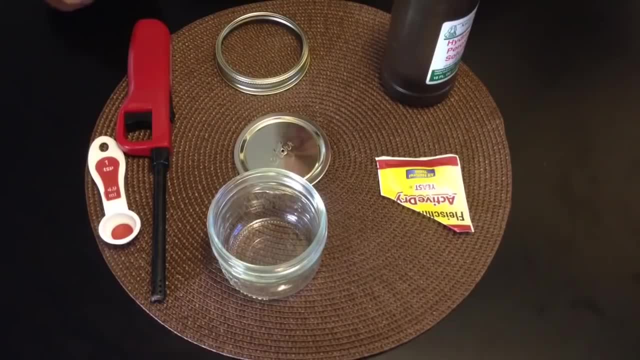 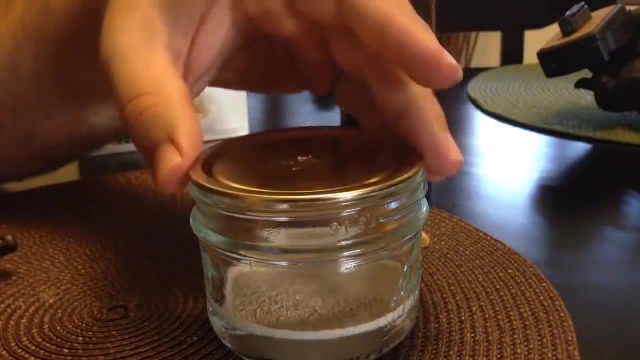 and poke a hole into the lid. that's about the size of the hole in your noodle. Not the entire noodle, just the whole of it In the small jar. fill about a quarter of it with hydrogen peroxide and half a teaspoon with dry yeast and try to tighten the lid by pressing on it. Shake it up to get the 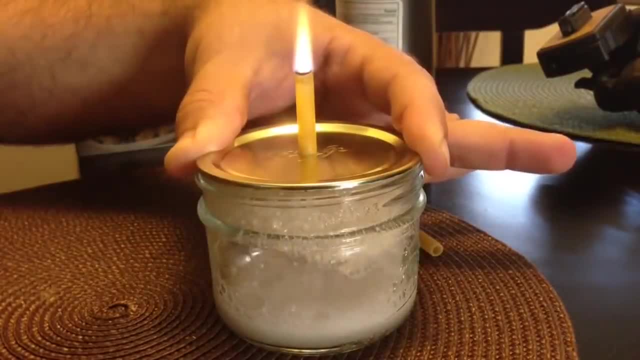 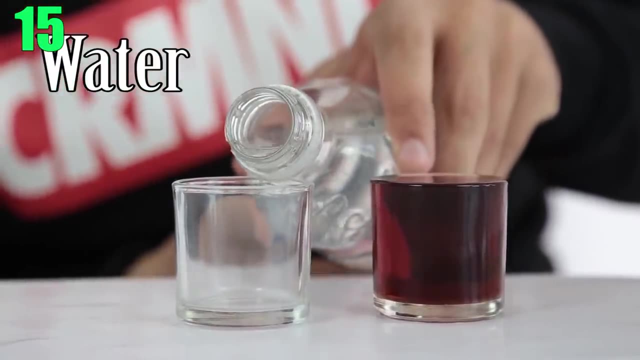 reaction started. Place your noodle on the lid and light it up. Now you have a miniature rocket engine. Number 15, turn water into wine. For this experiment you'll need two glasses that are the same: Wine water and something thin like a card or plastic layer. Fill both glasses at the. 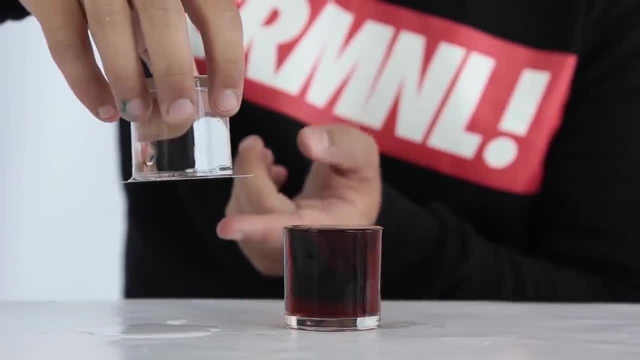 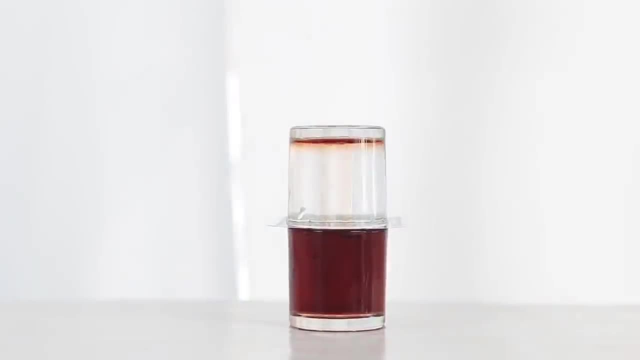 top one with water and one with wine and place your card over the glass of water. Apply pressure, sort of to get a little vacuum seal, and place the glass of water above the wine. Then gently pull the card until there's a small enough gap for the liquid to seep out. Eventually the wine will fully. 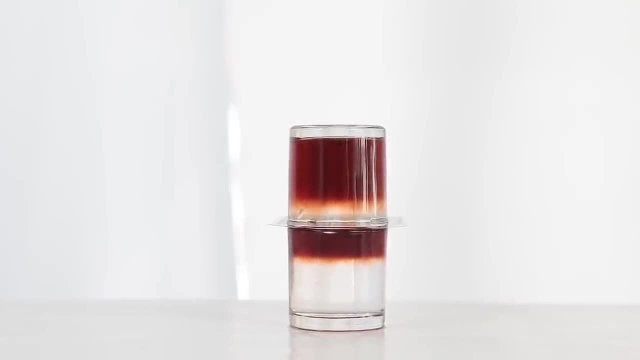 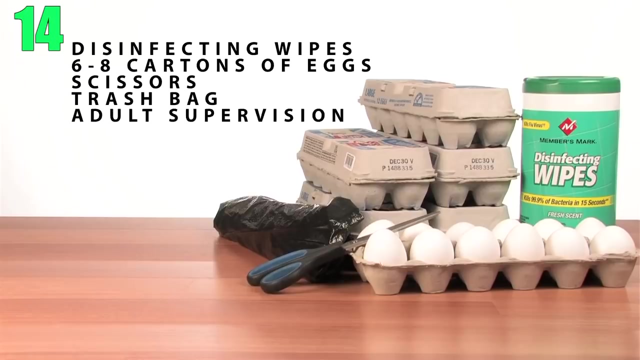 replace the water. Number 14, walking on eggs. Okay, so this is extremely wasteful, but pretty cool. Lay out however many cartons of eggs you wish in a path that you can walk on, but make sure they aren't cracked. 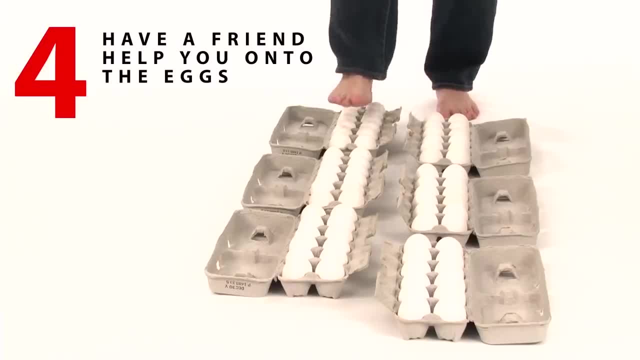 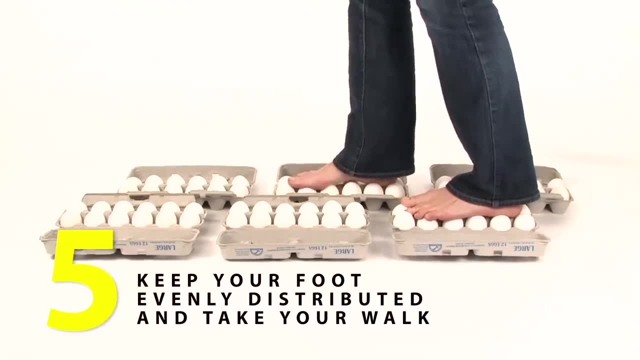 because you know, some grocery stores are a little bit snake like that. Then go ahead and walk on them. This is possible because it's very, very difficult to crack an egg on its edges and having a lot of them also helps. It also helps to distribute your weight more. The cartons of 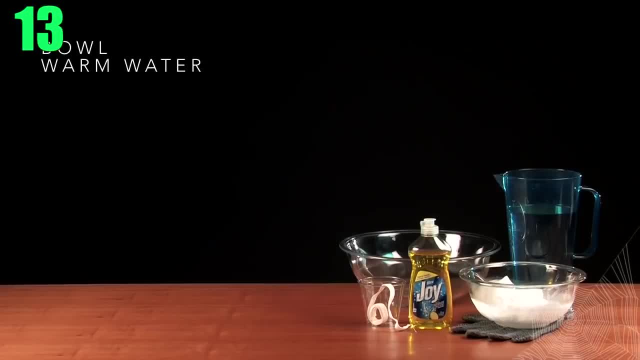 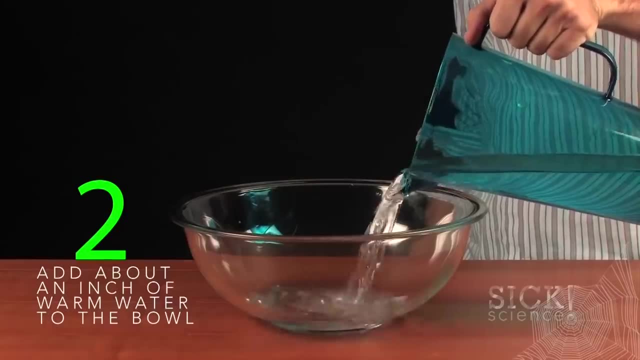 course they play a part in this too. Number 13, crystal ball. First, mix together about three parts water to one part dish soap to make a bubble solution. Then, in a bowl, pour enough warm water to get an inch of height Using a heavy-duty. 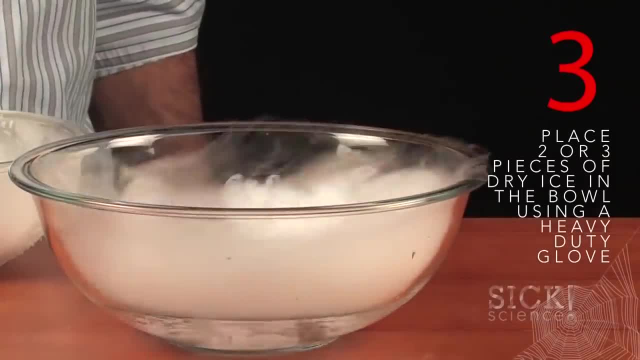 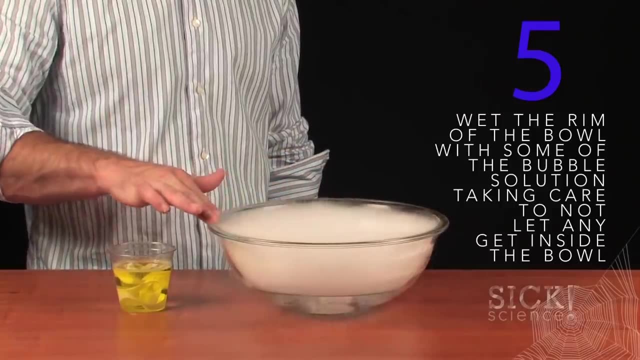 glove, which is important. place two to three pieces of dry ice into the bowl of water. Then dip your fingers into the bubble solution, wrapping it around the rim of your bowl to make sure not to let any fall in. Next, run a piece of long cotton fabric into a bubble solution and run your fingers. 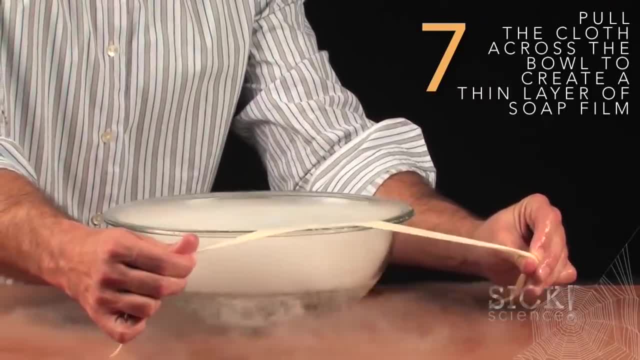 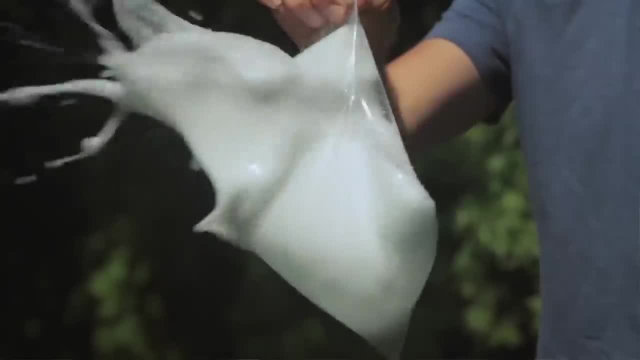 through it to remove any excess solution. Finally, run the cloth across the bowl to create the thin bubble layer. Then the dry ice will cause the bowl to grow and look like a beautiful crystal ball. Number 12,: exploding lunch bag. Start by filling up a Ziploc bag with half a cup of warm water and 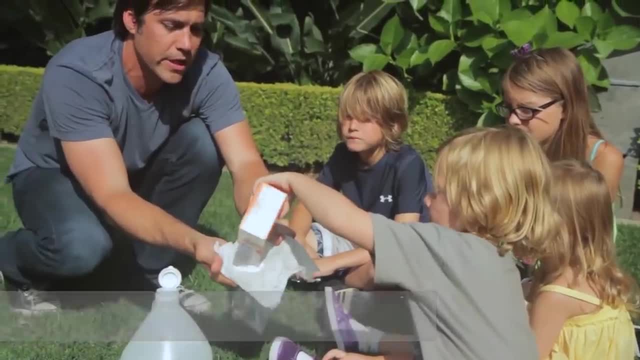 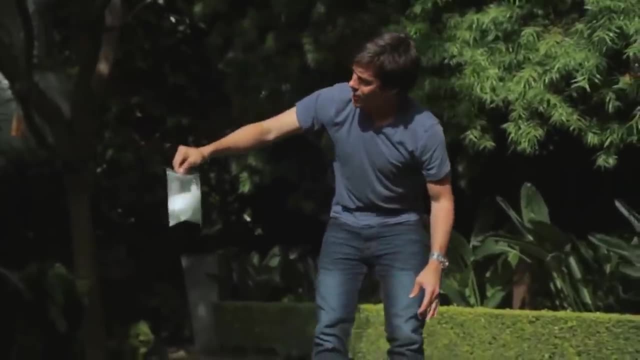 half a cup with vinegar. Then add some baking soda to a tissue. Make sure to wrap it up so none of it gets out of the bag right away. Now, while holding your tissue, seal the bag up nice and tight and let the tissue drop. Boom, Science baby. 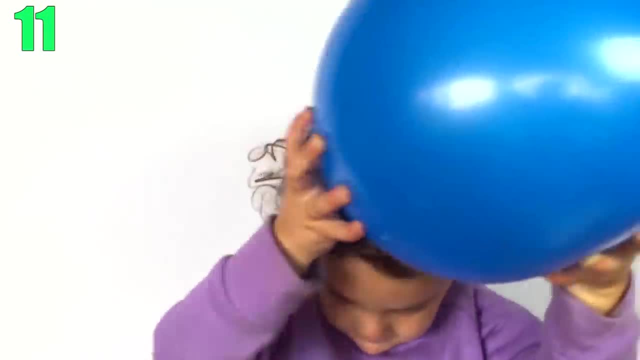 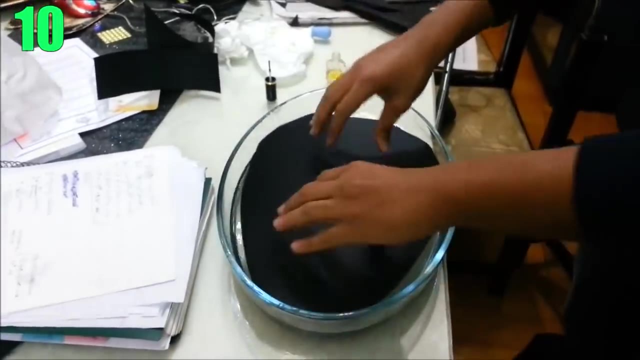 Number 11,: it can walk. Here's another trick that you can do with static electricity: Rub a balloon, put it on your hair or a towel, and you can manipulate a can into rolling whichever way you want. Number 10, rainbow paper. For this, we'll need a piece of black paper In a room with decent. 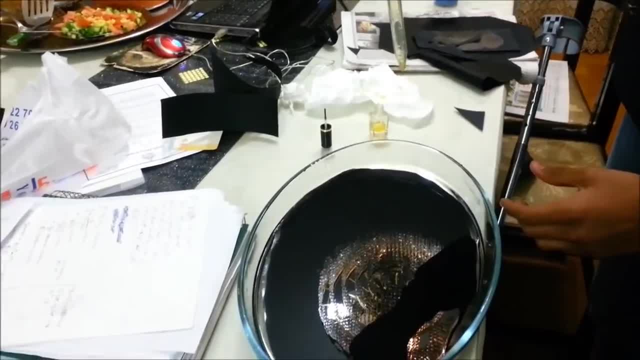 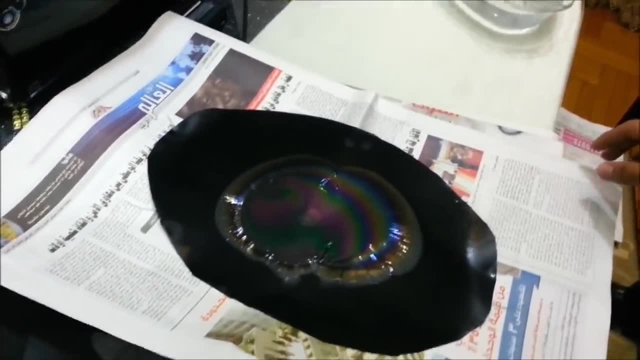 lighting. drop it on a container filled with water and use an eye dropper or something to slowly pour in drops of clear fingernail polish. Once the nail polish has dried, after a few minutes, pull out your paper and remove any water. Set it down on somewhere like newspaper to let the whole thing. 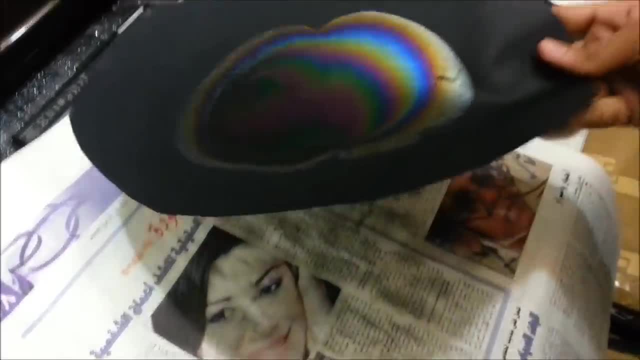 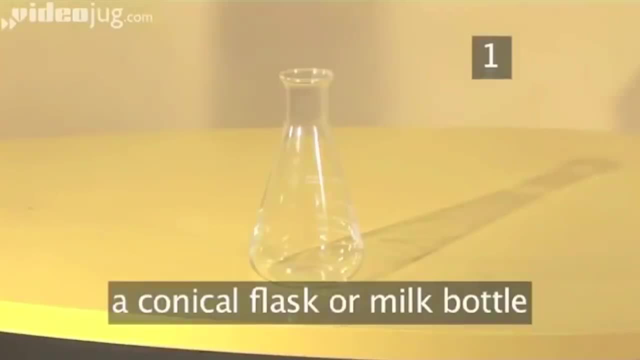 dry. Number 9, suck an egg. For this experiment, you'll first need a flask glass or container that's thinner than the egg at the top. Make sure your egg is hard boiled, by the way. Come on, I mean, we're not magicians. Next, set a piece of paper. 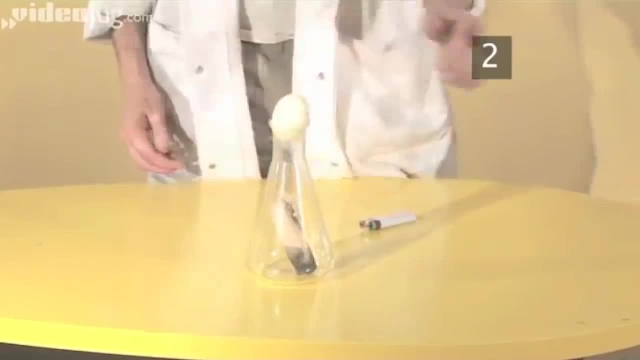 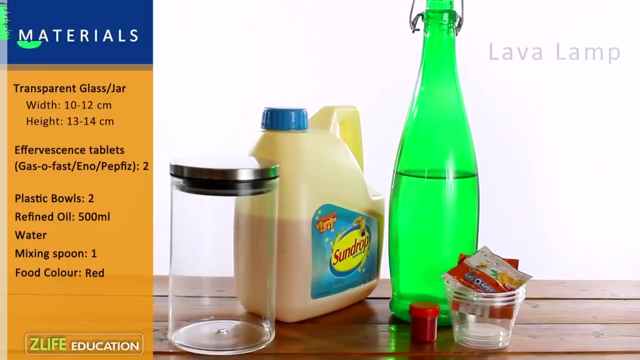 on fire and place it into your container. Place the egg onto the neck of your container and watch what happens. If you want the egg to come out again, just blow some air into it. and voila, Number 8, lava lamp. This one's actually lit. First, you'll need to fill a glass with one cup water. 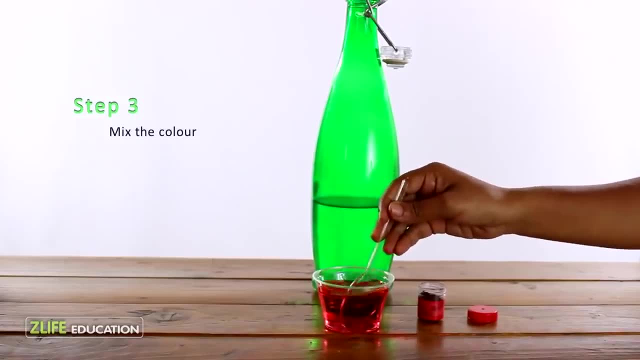 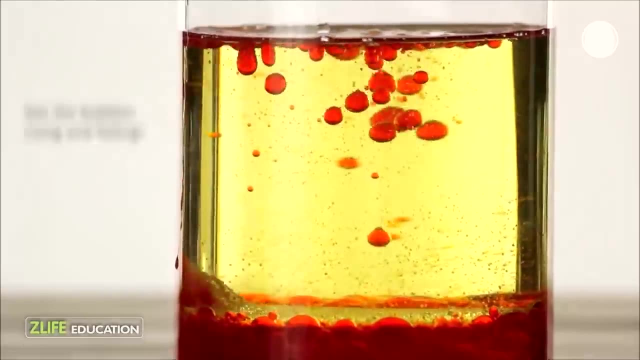 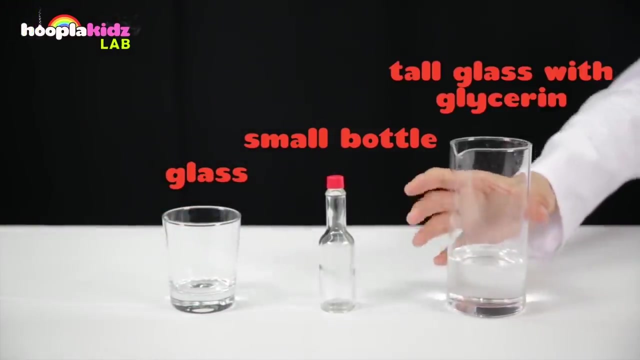 that you mixed with coloring, in this case obviously red. Then add three cups of oil into the glass gently so that it doesn't mix. Let it settle, then drop in either an effervescence tablet or Alka-Seltzer Number 7, invisible bottle. To do this experiment you'll need a glass, a smaller bottle and 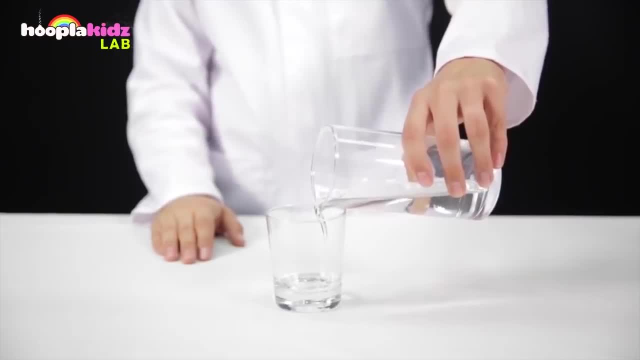 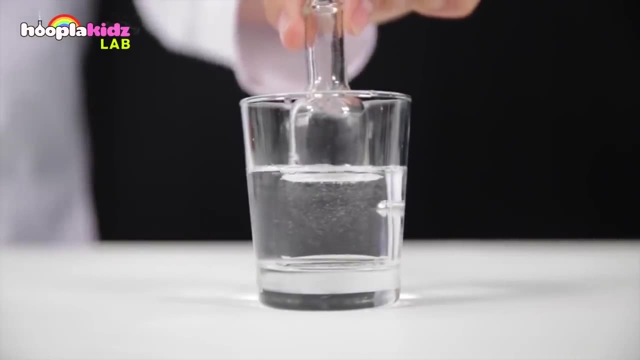 glycerin. Fill the glass with a reasonable amount of glycerin, then pour the rest into a bottle until it's close to the same height. Very carefully, place the bottle into the glass and boom, you can't see it anymore. This is because glycerin refracts or bends light, making it very difficult to see the 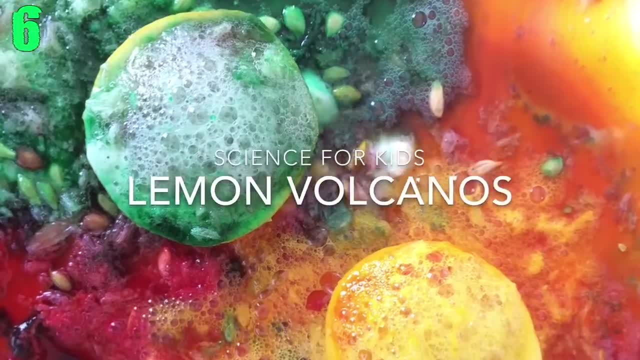 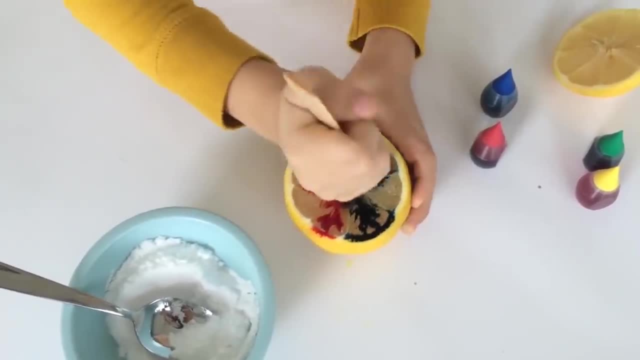 bottle Number 6,: lemon volcano. First you'll want to cut a lemon in half and in one half drip any desired food colorings onto the lemon and mix it in. Then add a spoon of baking soda and mix that in as well For a 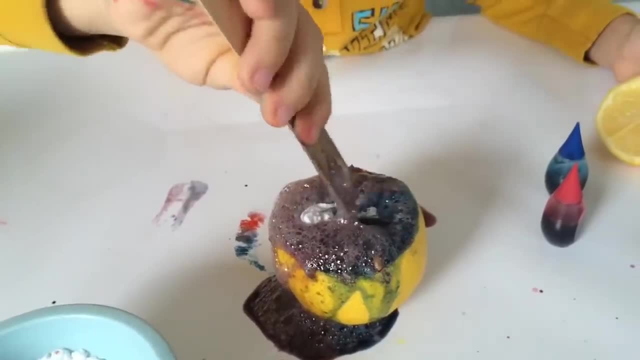 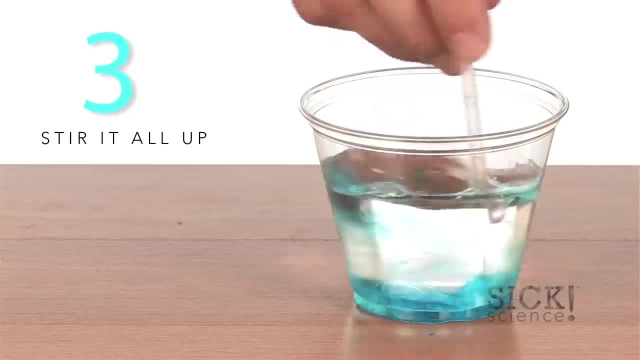 stronger reaction, squeeze the other piece of lemon over it. Number 5, bouncing bubbles. In a cup mix three parts water and one part dish soap. Then you use something to make a bubble like a wand, or maybe you can even use your hand to make a circle with your fingers. then 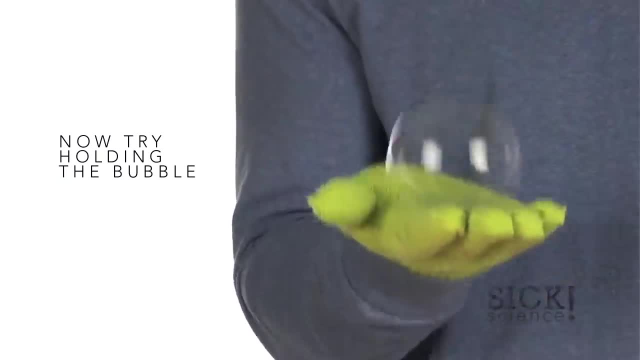 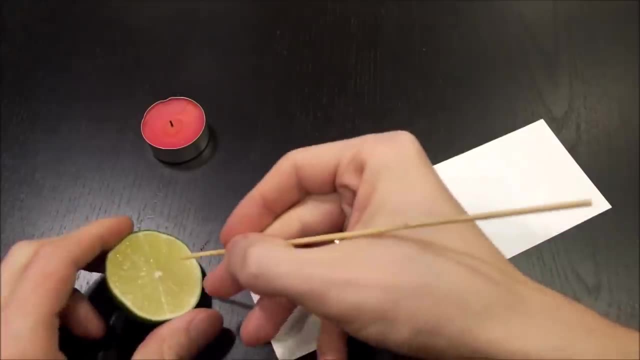 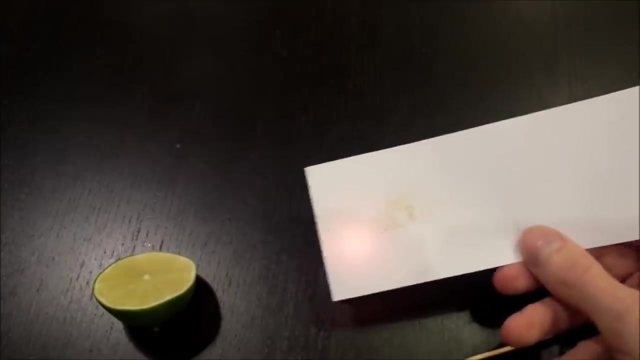 simply blow your bubble over your hand with the content. gloves on. Okay, this is going to be a little bit more tender now, Apparently. Number 4, invisible ink. First cut a lemon in half. then use either paintbrush or toothpick to take a bit of lemon juice at a time and write your message out on a piece of paper. Then use a source of light and heat, maybe a candle- and run your paper over it to easily reveal the message. 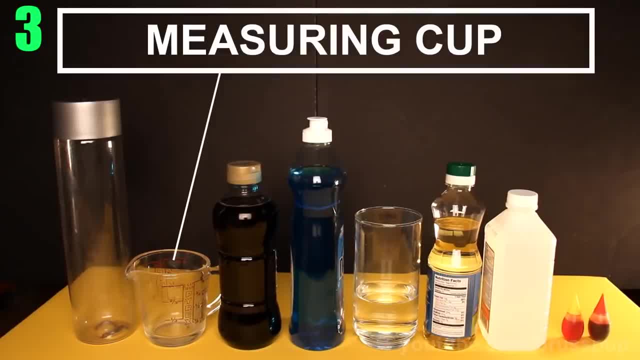 Number 3, liquid layering. So you know the saying blood is thicker than water. Well, it's true, of course, but to the point that some liquids have higher densities than others, which you'll see here. What you can use is an empty bottle, something tall, a measuring cup or a paper towel. 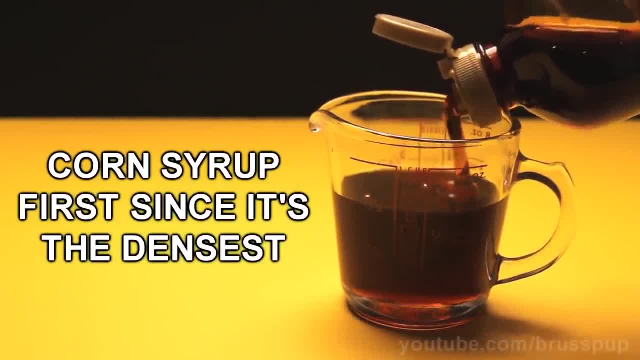 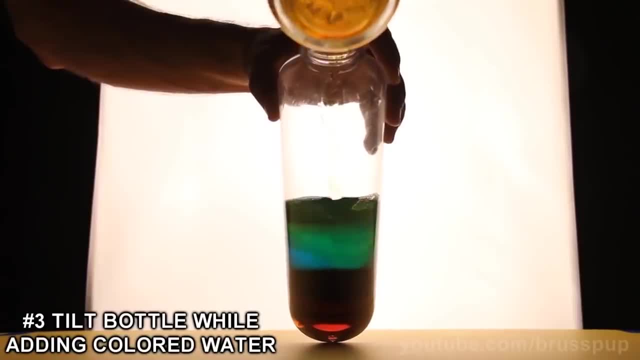 up Dark corn syrup, dish soap, water, vegetable oil, rubbing alcohol and food coloring to mix with alcohol. Measure how much your bottle can hold by ounces or millimeters and divide by 5 because of our 5 liquids. Then pour each one in carefully into the bottle in the way. 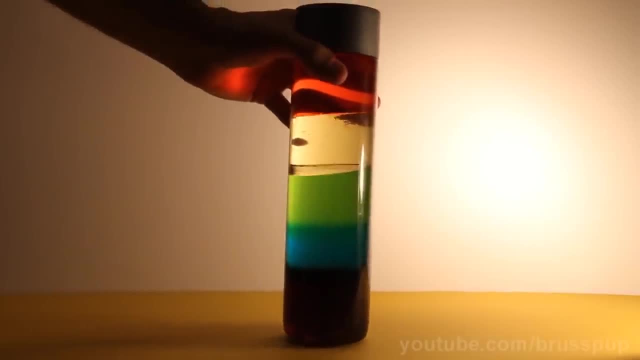 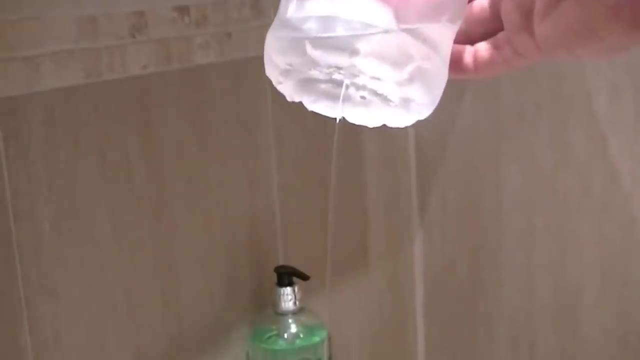 we listed. So corn syrup first and alcohol last. Looks pretty cool, right. Number 2. Waterbending. For this you'll need running water, either from the tap, or you can have a bottle of water with a hole in it. Either way, just have the water running. 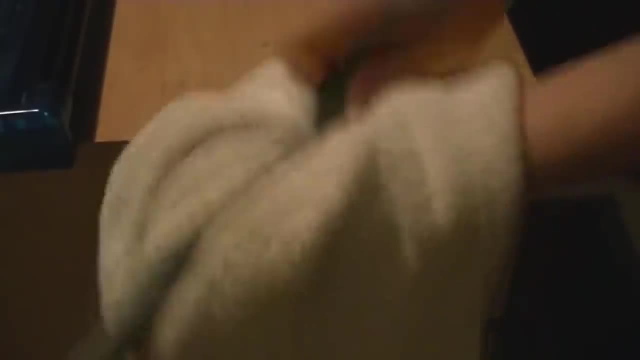 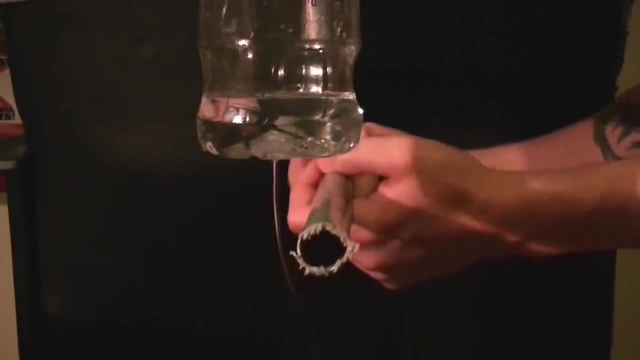 gently. Next, you can either use a PVC pipe and a towel or just run a comb through your hair, but we're trying to get a static charge here. Then just play around with your pipe or comb near the running water and you can control which way the direction pours It's.